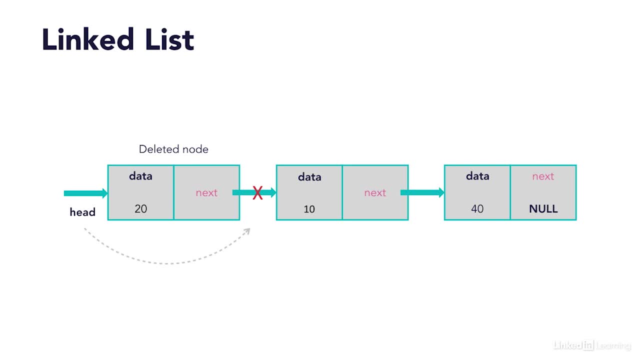 anything Unlike an array, where you have to statically set the number of elements you need. a linked list is a great alternative because you can link them dynamically, allowing your list to grow or shrink as needed. To create a linked list, we first need to create. 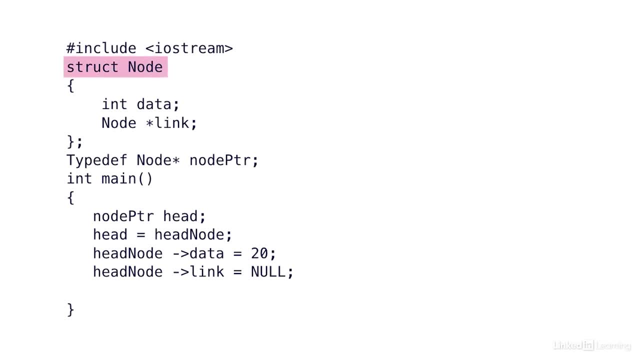 a struct or a class. I'm going to use a struct. I've defined my struct as node In my node. I have a data point and I also have a pointer, a pointer to another node. This line, node asterisk link, is a pointer to a node. The line after that, typedef, node asterisk, is: 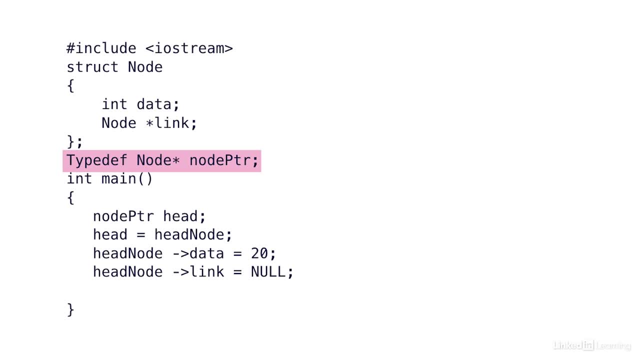 redefining what node pointers are. So instead of having to require an asterisk anytime I use a pointer, I can now just declare them as type node pointers. It's the same thing. You can use typedef anywhere you need, but it's highly recommended to only use them when needed. 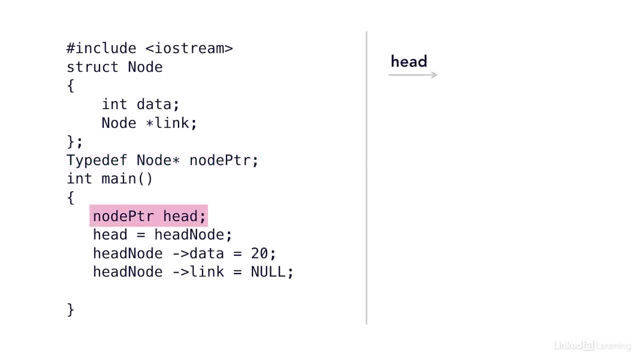 So in my main I have node pointer head. This creates a new node pointer called head. Right now it's not pointing to anything, but we'll get to that in a minute. The next line says: head equals asterisk, Head equals new node. So now I'm going to point to a brand new node And remember every. 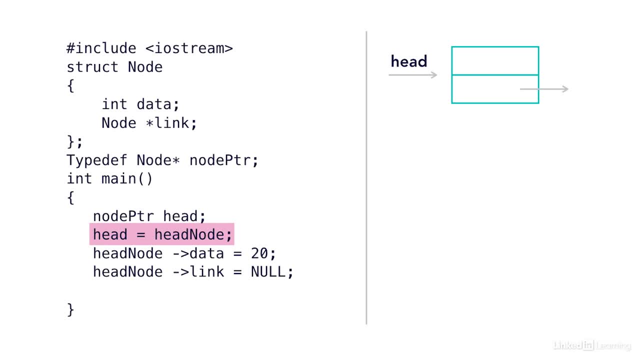 time I create a node, I get the same data points that are defined in the struct node. So I have an int data section, which I've defined in blue, and then I have a node pointer. Right now again, it's not pointing to anything. The next two lines populate my new node with: 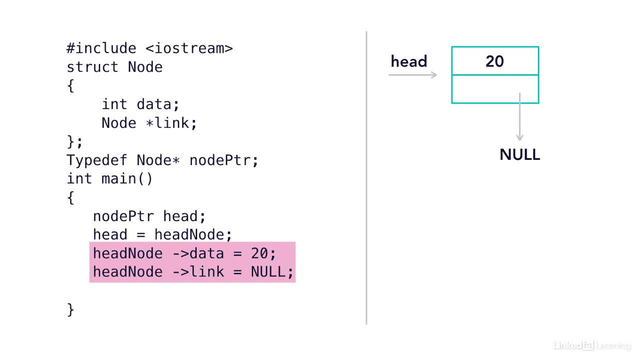 data. We're also introducing the arrow operator. This is used when you're using pointers in reference to data, To populating data. So here I have my pointer head pointing to a new node, And now I want to put 20 in the data spot. I'm also pointing the link portion to null. Next line is just: 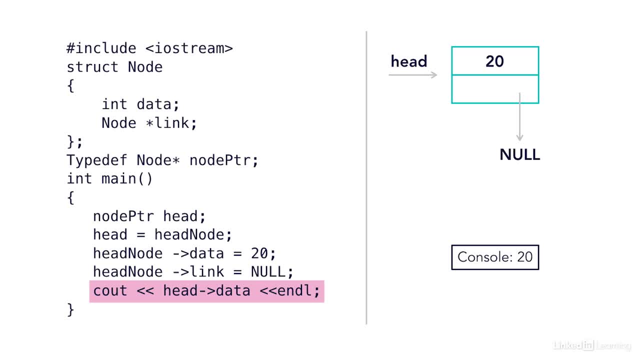 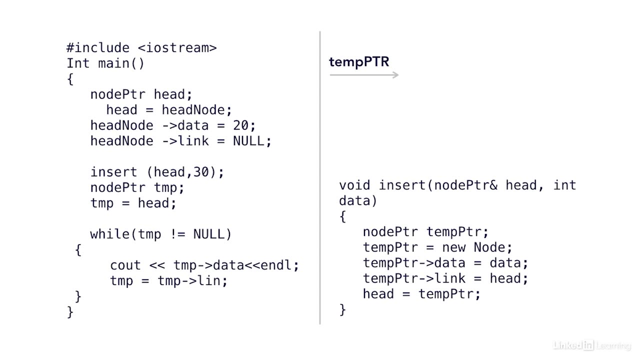 for data debugging. If I try to print out the data that my head is pointing to, it should give me a 20. So all I need to say is head arrow data And that will get the data that the head pointer is pointing to. But what if we have more data? What if we want to insert? 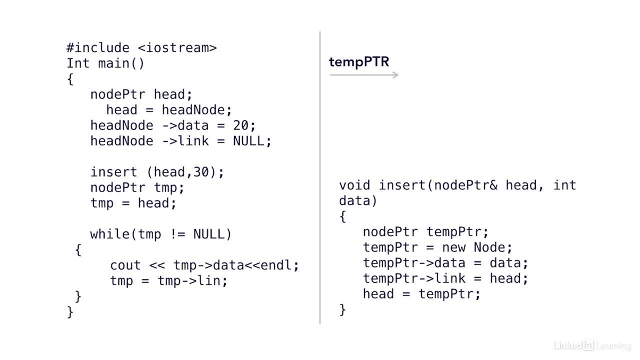 a whole bunch of data into our list. Here I've written an insert function. It requires a pointer- pass by reference- Remember, pass by reference versus pass by value- And a data point And it'll take that data point and populate a new node. 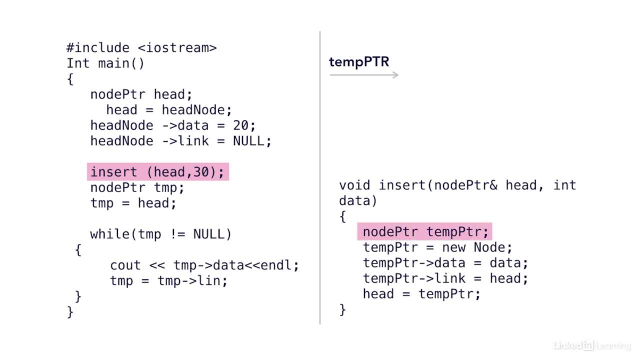 So the first line in my function declares a new node pointer called temp pointer. I've named it T-E-M-P-P-T-R for short. All that does is create a new pointer. Currently it's not pointing to anything. The next line creates a new node and makes the temp pointer point. 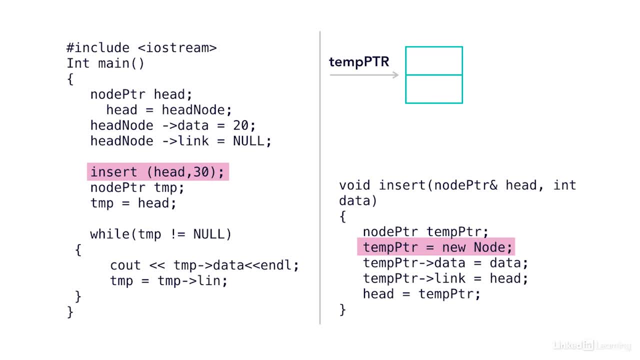 to this new node. So now I have a brand new node. Anytime I declare a node, I get the same two pieces of data: An integer for the data type and then a link for the next node. I populate my data. I put 30 from my parameter list. 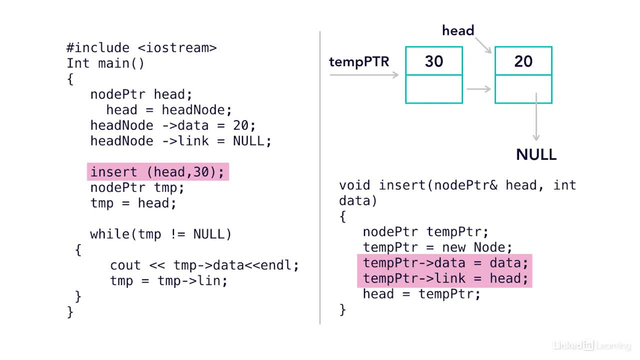 Into the data portion And then the next line says temp pointer link. So now I'm linking the next node to head. So remember our head was pointing to a node with 20 in it. So now I have two pointers pointing to the node with 20.. The last line redirects head to the front. 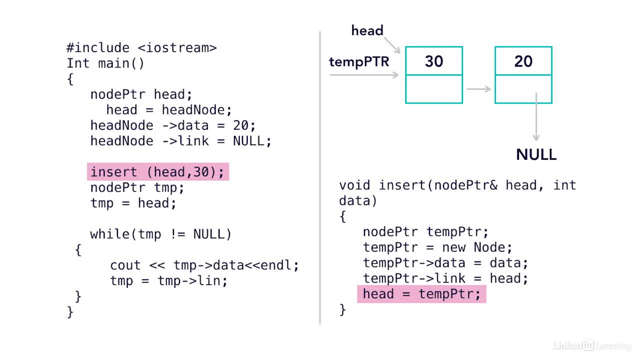 of my list Head should always be the front of your list. It makes it easier to find the start of your list, So I can either insert a list into that empty list or where to start searching and sorting from. So now my head is pointed back around the same place. my temp pointer is pointed to 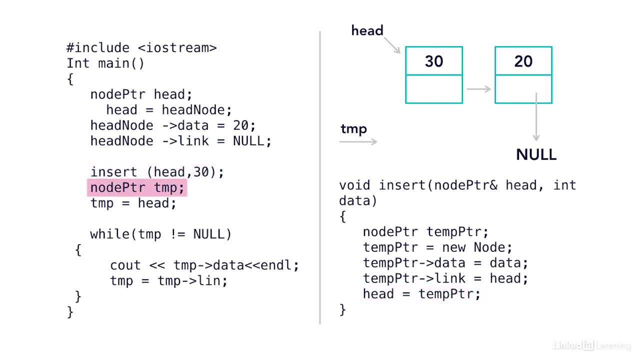 which is the node that has 30.. As soon as I return back from my function, temp pointer will be deleted Because, remember, it was only created in that function. So now my list only contains a head pointer pointing to the node with the 30.. 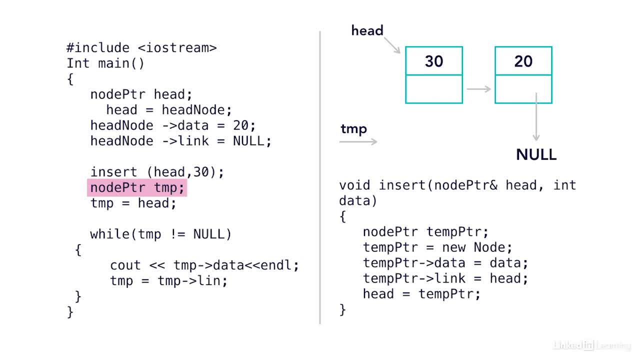 The node with the 30 pointing to the next node with the 20.. and the node with the 20 pointing to null. We could keep inserting, but let's print out our list. So when I return back from my function, the next line creates a new temporary pointer. 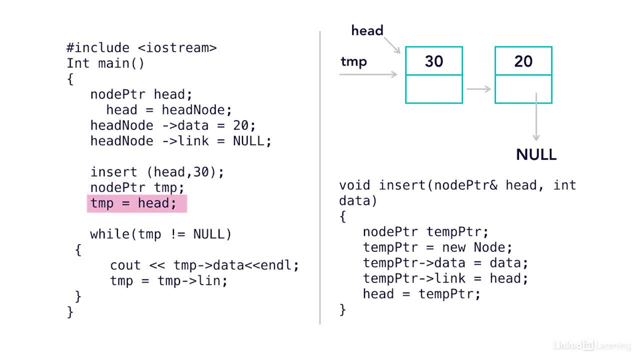 currently not pointing to anything. Then I set it to point to the same place as head. Head should be at the front of my list. And now I say: while temp or that pointer is not equal to null, So while I'm not at the end of my list.